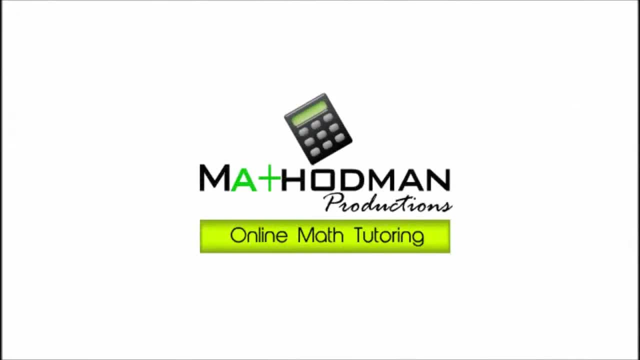 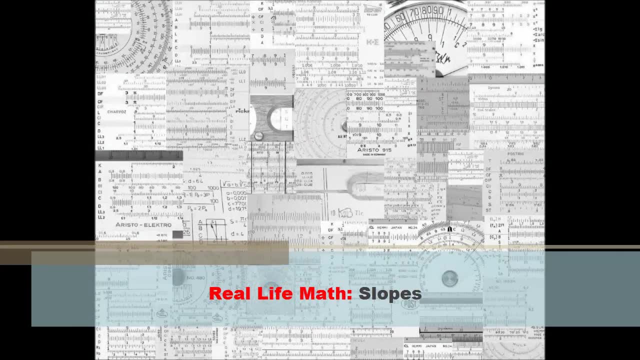 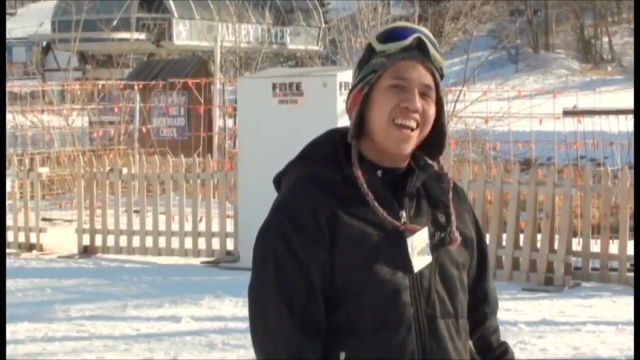 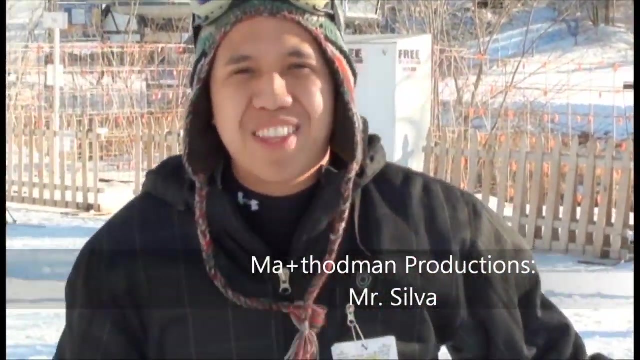 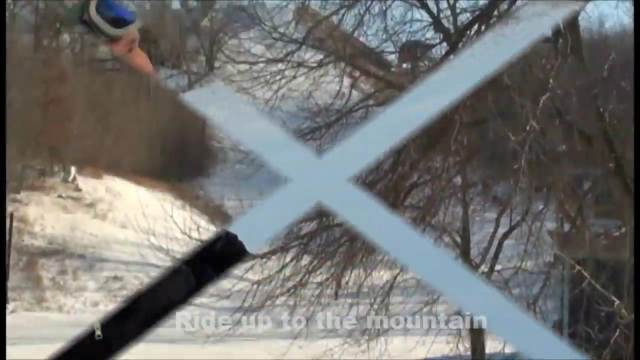 Oh hey, Welcome to Real Life Math. I'm your host, Mr Silva. Today we're going to take math to the extreme. You know how? We're going to learn about slopes? by hitting the slopes. How are you feeling? I'm feeling alright. I'm not too scared. I've gone two or three. 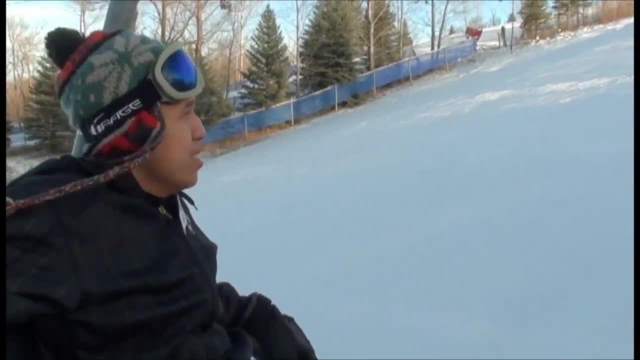 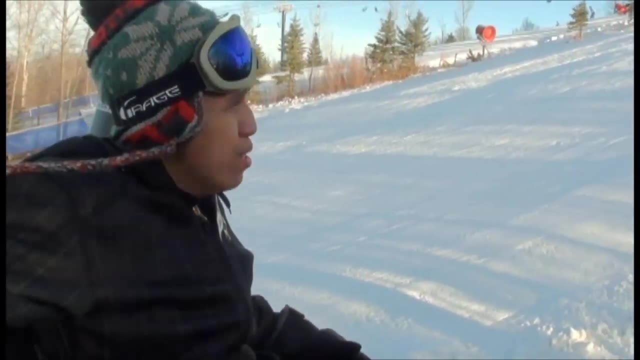 times. Let me tell you a little history about this mountain. See, back then Chuck Norris himself came to this exact same ski lift. You know what happened to him, What He had to be escorted down because he was too scared to go down the mountain. But I'll be alright. 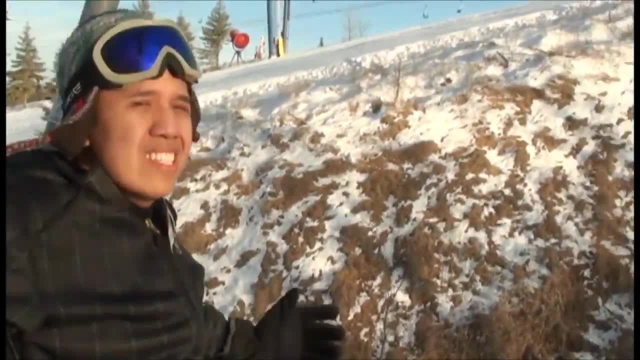 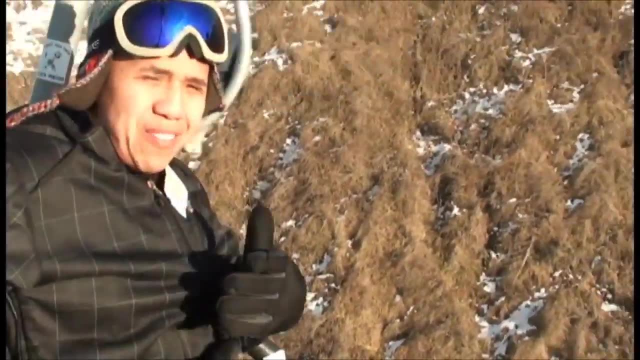 Back then in high school, you know what they used to call me: The guy that got dumped twice on Valentine's Day. I'm not going to bring that up, man. They used to call me the Silva Surfer, you jerk. This winter, my good friend and I went down to Wisconsin Alpine Valley. 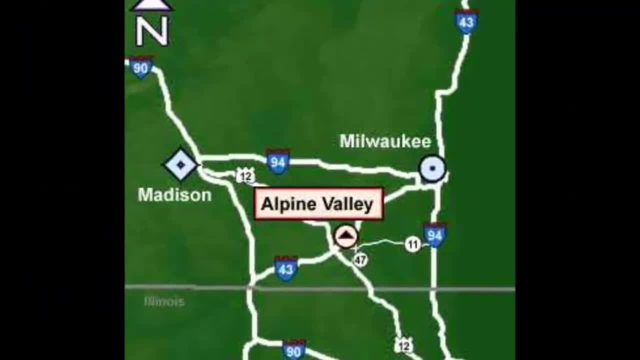 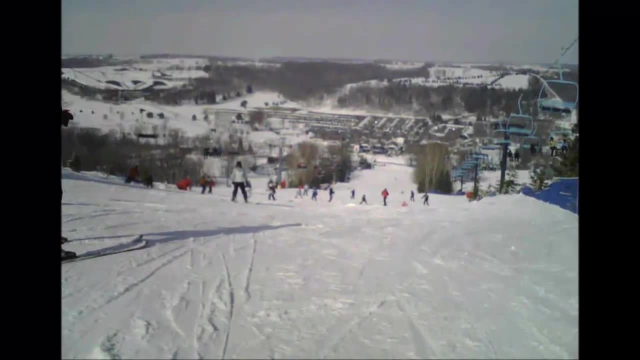 to go snowboarding. I've only gone two or three times, so he didn't think I could do it. I bet him a meal that I can beat him faster down the mountain. So what do you guys think won? Let's find out. 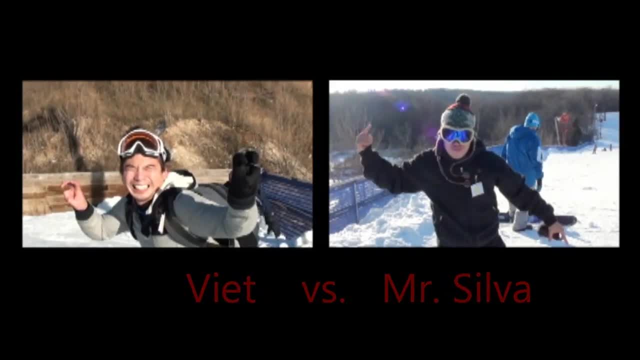 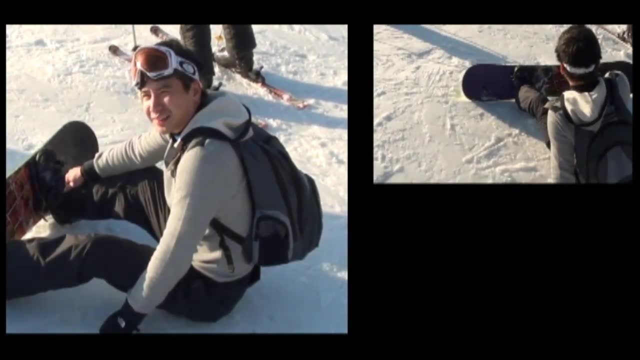 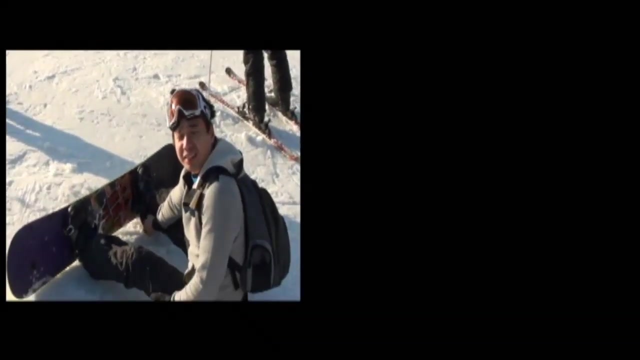 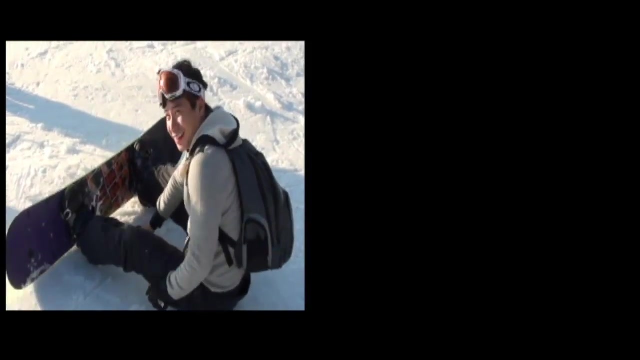 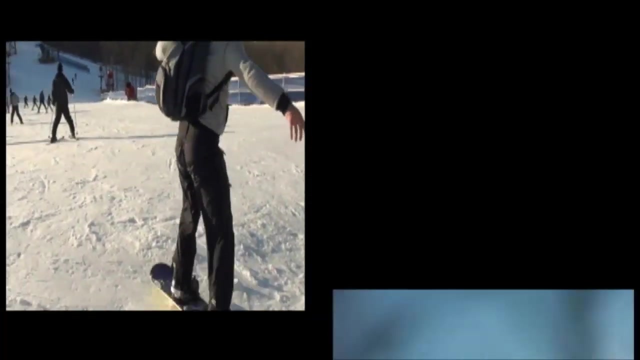 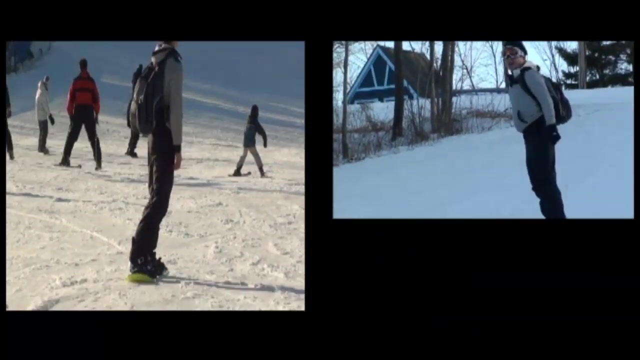 You ready to get beat? Can I help you Now? watch me What I do Now. thank you for coming to my drive-thru. You know what I mean. All right, before you go down the mountain, snowboarding is a great way to get up. You can do it in fishing, in snowboarding, in the woods, you can go. 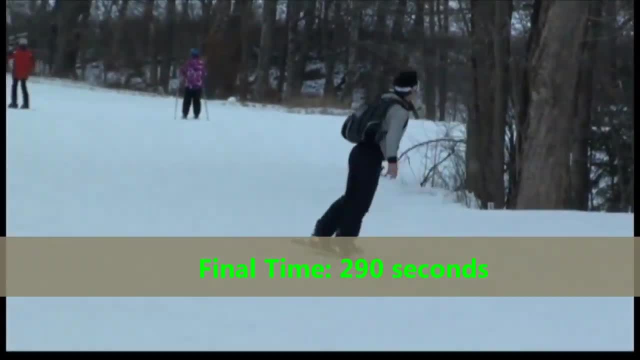 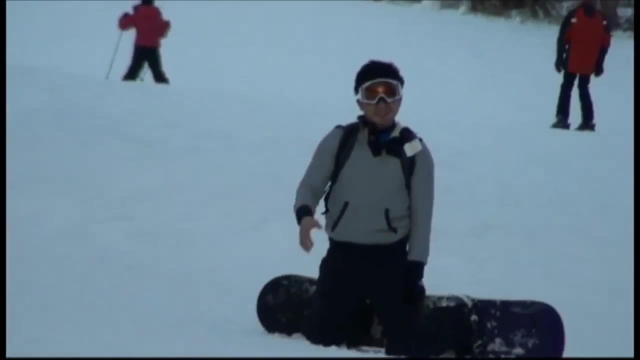 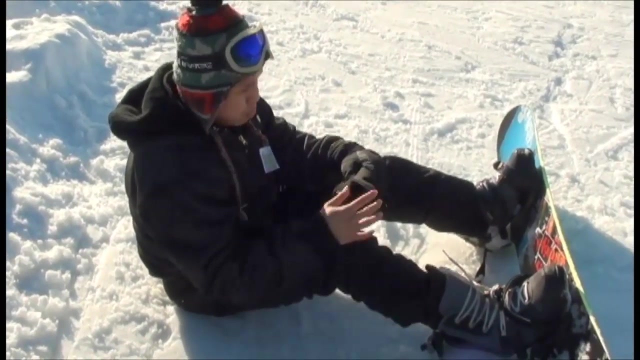 boating, you can swim. You can do anything you want to do in your life. You don't have to worry about the coronavirus. You can go down the mountains. You can go out and go. Snowboarding is very dangerous. Remember, always wear protective gear. 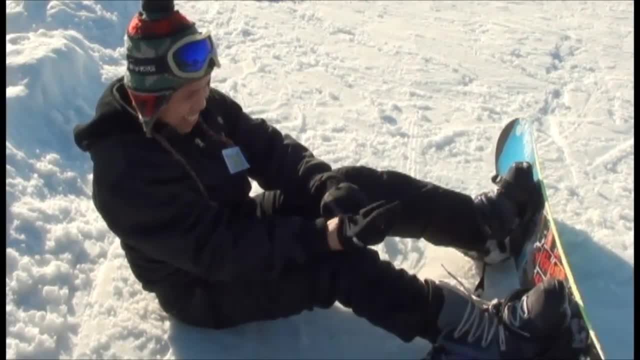 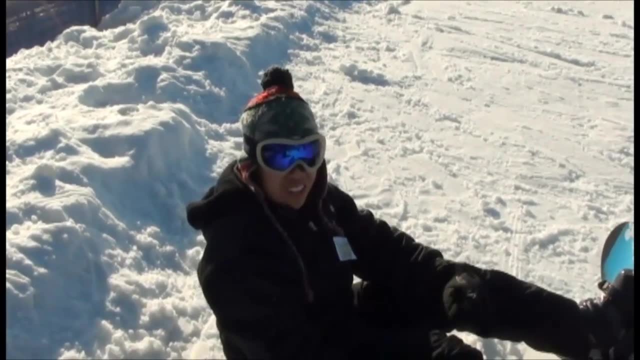 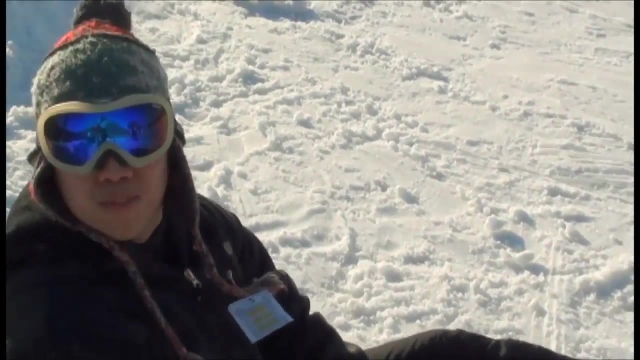 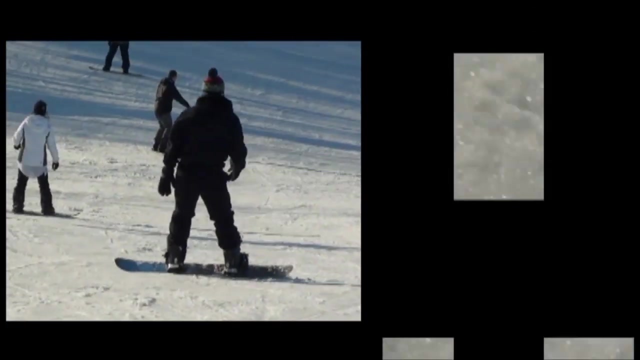 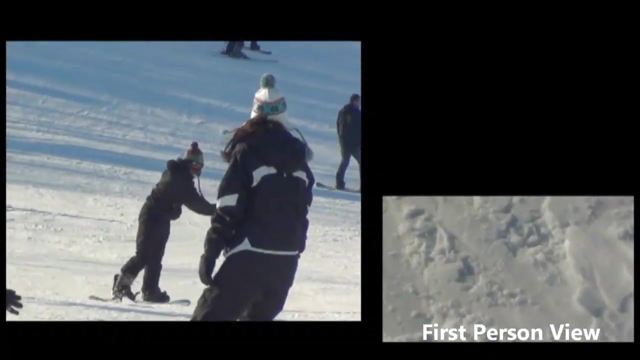 have your gloves on and have your cool-looking sunglasses on. Oh no, Make sure, the most important thing is to make sure you have your cool snowboarding gear on. Oh no, Anyone else see that. Oh, Oh, Oh. 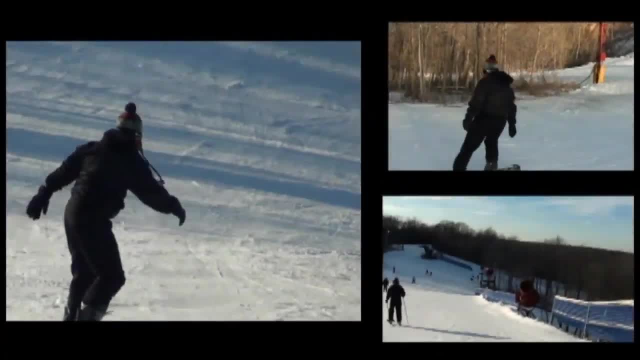 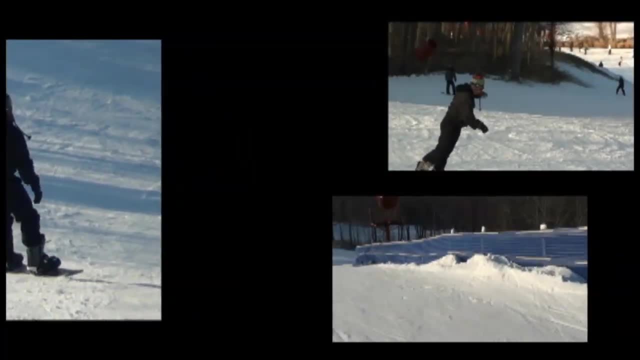 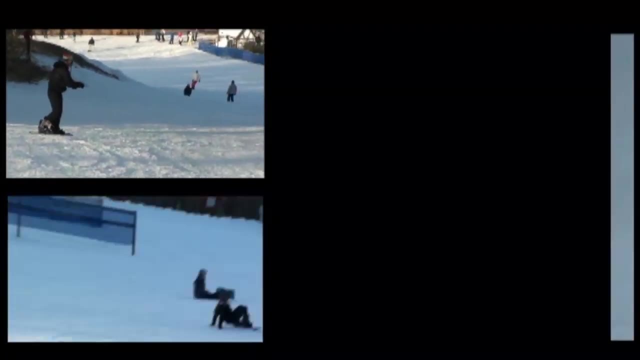 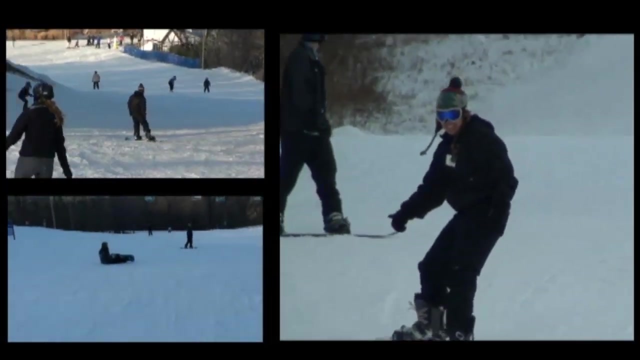 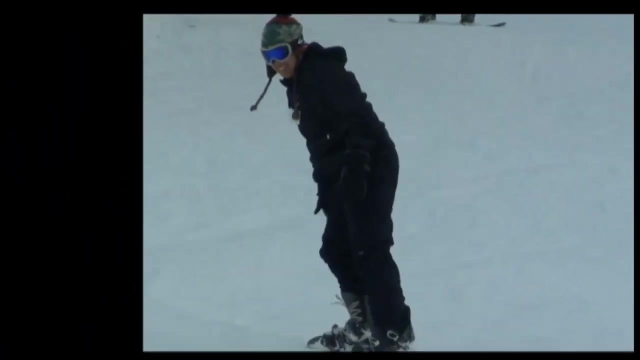 Steve, don't run into me. Good job Bam. He's breaking no speed limits. Never got a ticket in his life. Yeah, Oh, it's a snail, It's a tortoise. No, it's Mr Silva. 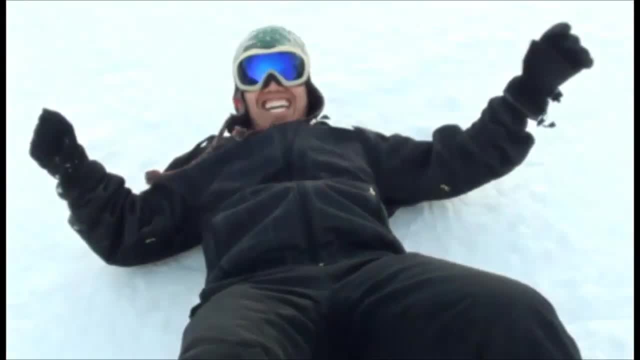 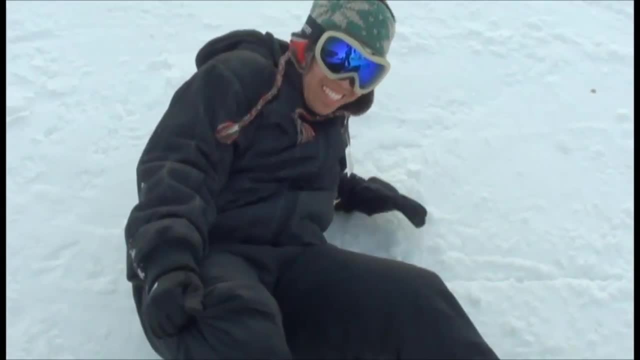 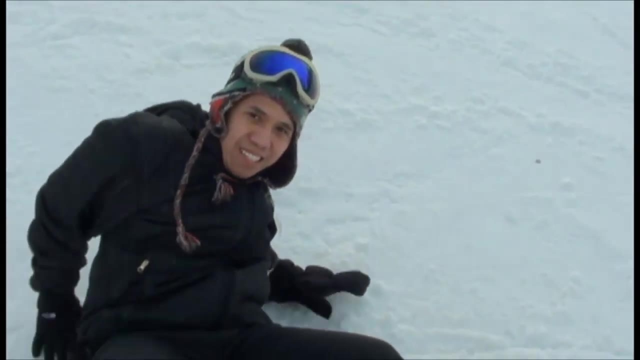 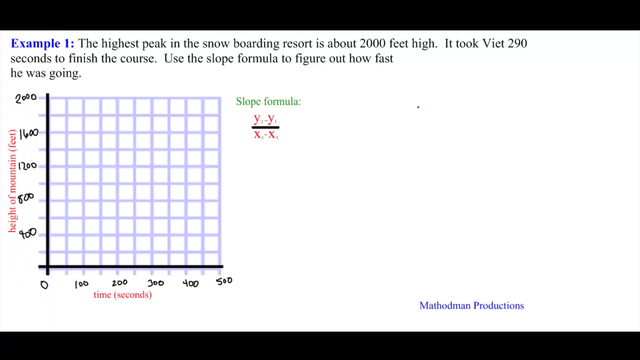 Snowboarding. Oh, John, Did I beat you? No, I'm close. I think I just had a birthday Shut up. Let's now take our results and relate it to slopes. The highest peak in the snowboarding resort is 2000 feet high. 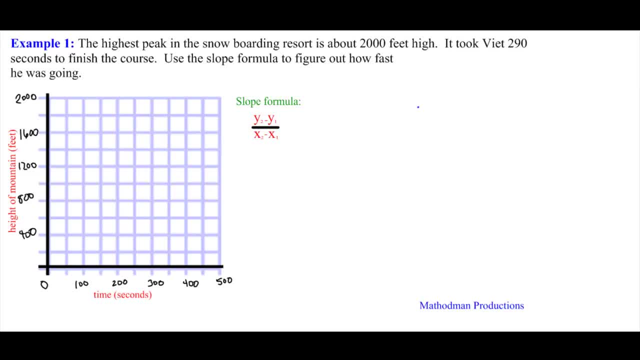 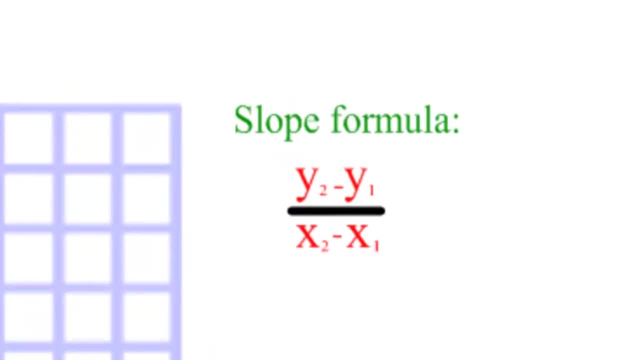 It took Viet 290 seconds to finish the course. Use the slope formula to figure out how fast he was going. In order to use the slope formula, you need two points. The word problem doesn't state it plain and simple, so we gotta look for those two points. 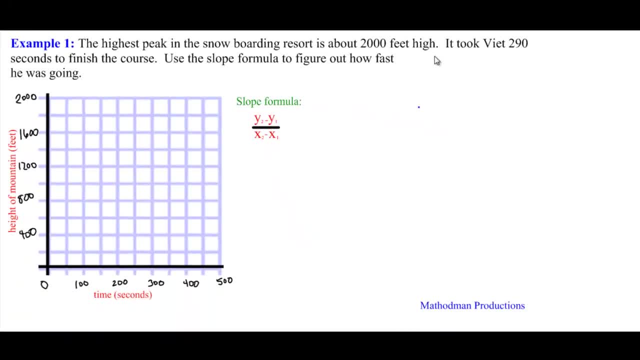 by just gathering up information. The first sentence says Viet was on top of the mountain, which was 2000 feet high. Let's mark our first point right there: In the top of the mountain. he didn't go yet, so that's zero seconds and that's 2000 feet. 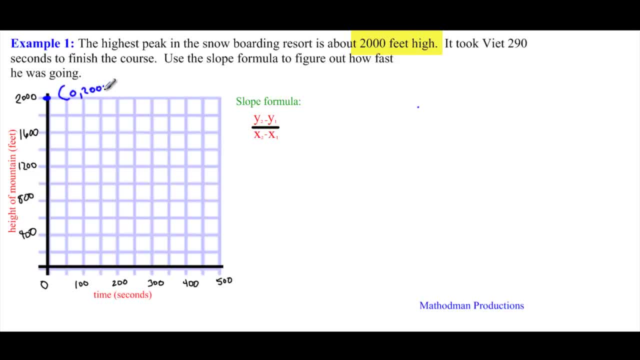 high- I'm just gonna write the coordinates right here. And as he was going, the whole course took him 290 seconds to finish. so when he's at the bottom of the mountain, or zero feet, Took him 290 seconds. That's our second point. 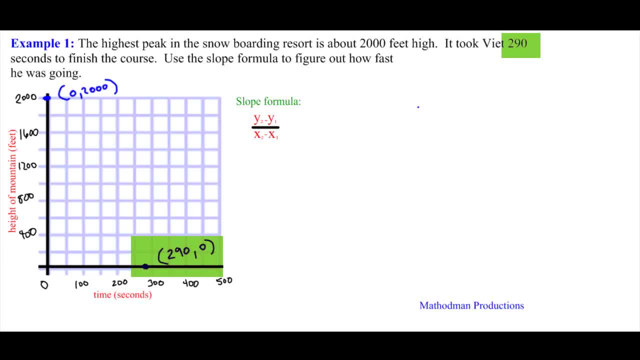 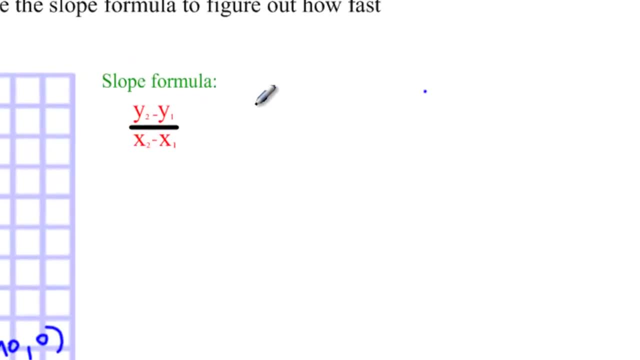 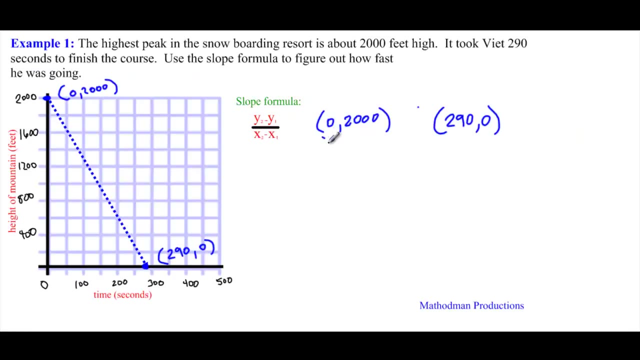 Two ninety and zero. Now that I have two points, then we can use the slope formula to figure out the rate that he was going down that mountain: Zero, two thousand and two ninety zero. I always like to label my coordinates first before I plug it into the formula. 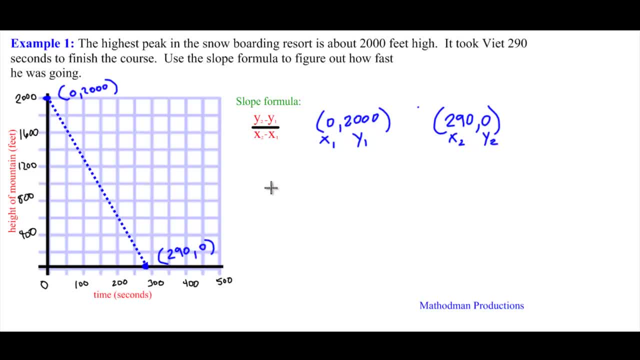 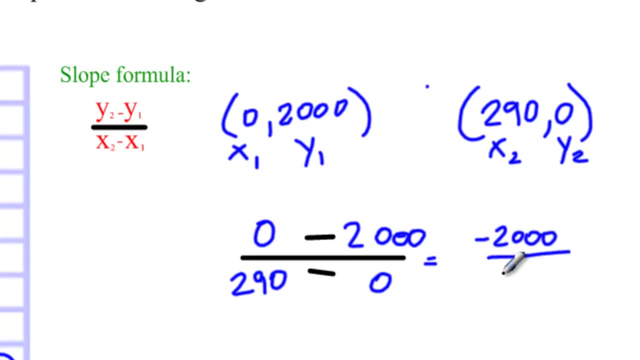 That way, all I have to worry about is putting the numbers in Into where they belong: Y two is zero, Y one is two thousand And x two is two ninety minus x one, which is zero. That simplifies to negative two thousand over two ninety, which is approximately negative. 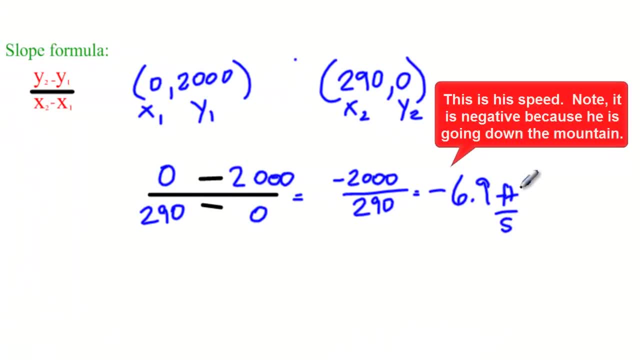 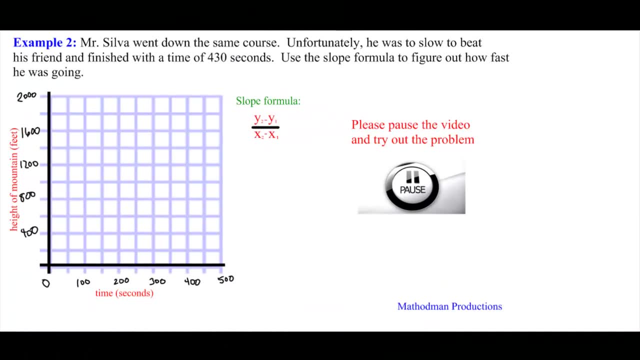 six point nine feet per second. My answer, Sample two, is very similar to the first example Here. Mr Civil went down the same course. Unfortunately, he was too slow to beat his friend and finished with a time of four hundred thirty seconds. 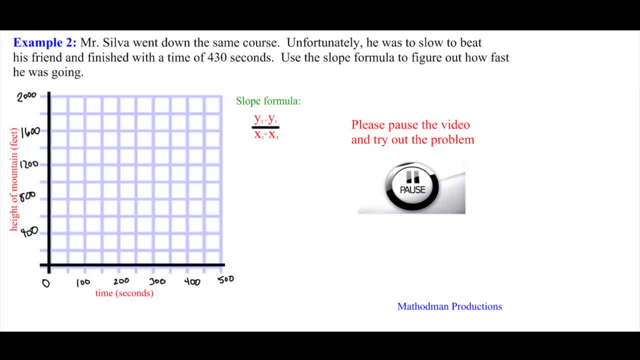 Yeah, I know I lost. You don't have to rub it in, It was still a lot of fun. I ended up owing my friend a meal, but it was only ten bucks, so not a big loss on my end. Moving on with the problem. 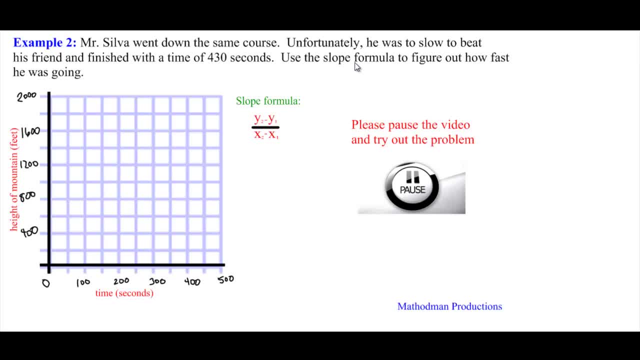 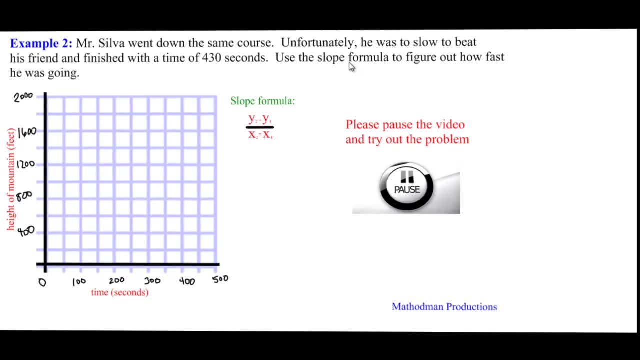 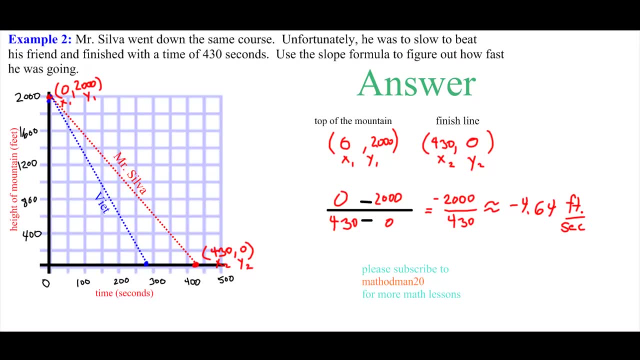 Use the slope formula to figure out how fast I was going. Please pause the video and try it out When you have finished. Unpause the video and your answer will be right in front of you. Here is the answer from the example. Remember to use the slope formula. you need two points. 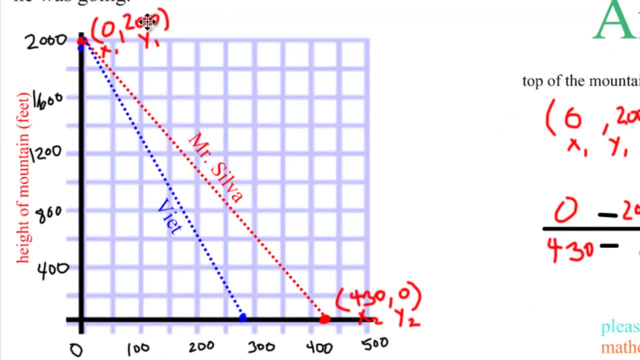 I started at the same spot in the mountain, which was two thousand feet high. So that's my first point: Zero and two thousand. My second point was at the bottom of the mountain, which took me four hundred thirty seconds to get to. So my second point is four thirty and zero. 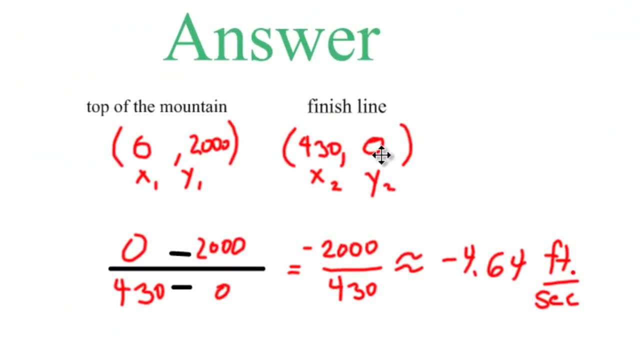 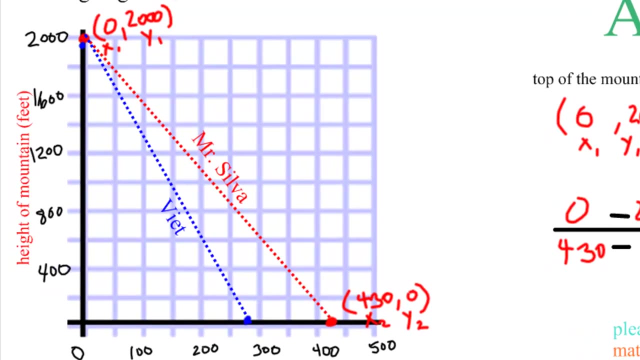 Okay, Now that I have two coordinates or two points, all I have to do is plug the numbers into the slope formula and I get the answer of negative four point sixty four feet per second. Before I end the video, I just want to point out a couple of things.